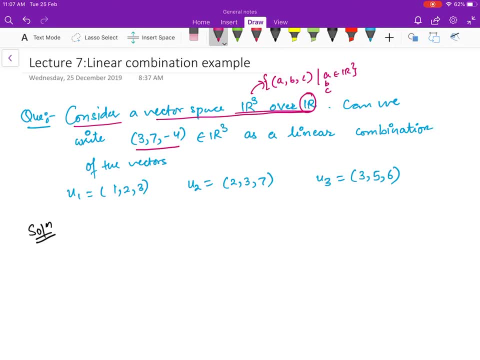 So the question is: can we write 3,7,-4 as a linear combination of these three vectors: 1,2,3,2,3,7 and 3,5,6. So this is your problem. So let us see how we can solve it. 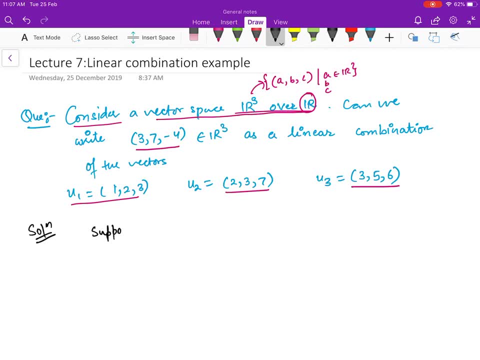 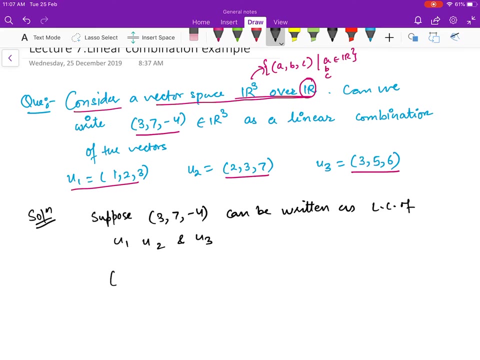 Now suppose 3,7,-4 can be written as linear combination of U1,U2 and U3. It means that you can write as: 3,7,-4 equal to some constant alpha 1, or you can just write it in the form of xyz. 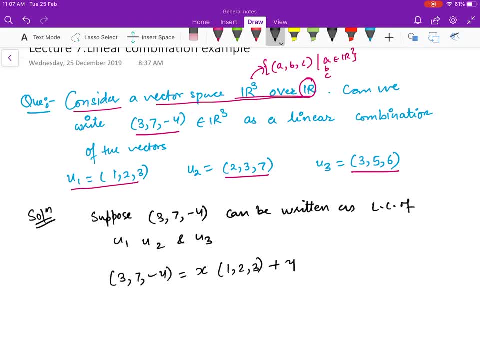 x is a real number, 1,2,3, plus y times, which again is a real number, 2,3,7, plus that time, which again is a real number, 3,5,6.. So you see, by definition, this, this and this, they are the real numbers and this is the definition of linear combination. 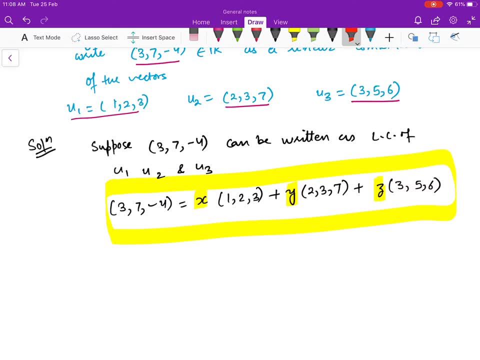 So this is what we mean by when we we say that 3,7,-4 is a linear combination of 1,2,3,2,3,7 and 3,5,6.. So this is what we mean by when we say that 3,7,-4 is a linear combination of 1,2,3,2,3,7 and 3,5,6. So from here, you know, by the operation, this is equal to 1 into x, 2, into x,3, into x, plus 2y,3y,7y plus 3z,5z,6z. you know, by the operation, this is equal to 1 x 2, 3 x, 3 y, 2 y, 3 y, 7 y, plus 3z, 5z, 6 z. so this should be equal to 3y6,7,6,6 and 3,5,6. 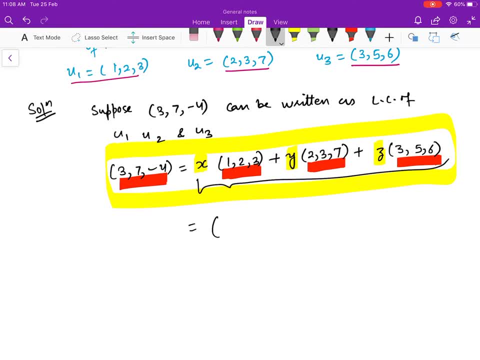 you know, by the operation this is equal to 1 into x, 2 into x, 3 into x plus 2y, 3y, 7y plus 3z, 5z, 6z. so you have this x plus 2y plus 3z, and then you have 2x plus 3y plus 5z, and then 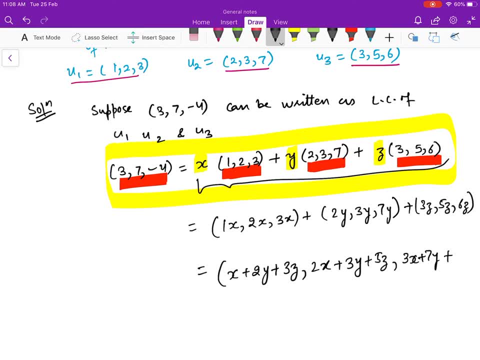 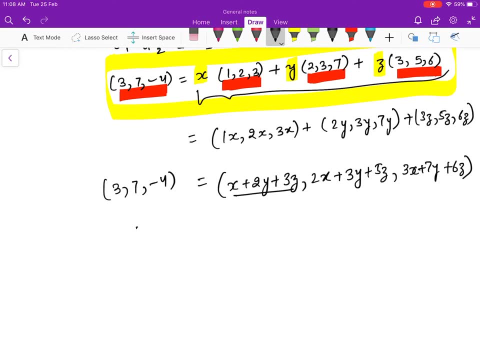 you have 3x plus 7y plus 6z and this is equal to 3 comma 7 comma minus 4. so component wise, you just equate. so you have x plus 2y plus 3z is equal to 3, 2x plus 3y plus 5z is equal to 7 and 3x plus. 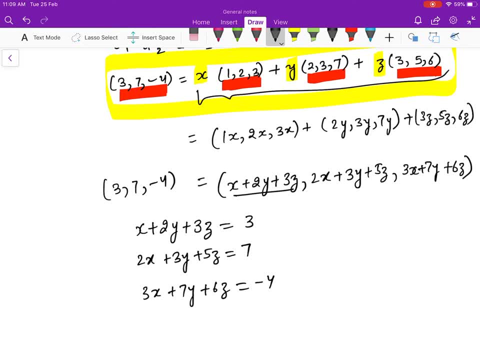 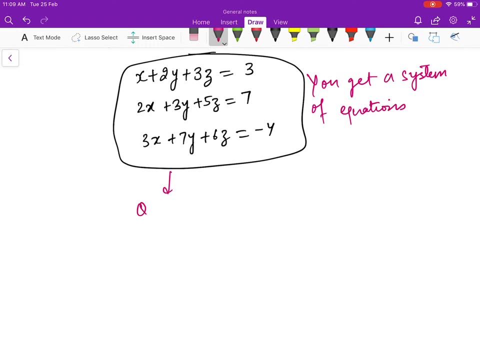 7y plus 6z is equal to minus 4. now you get a system of equations. you get a system of equations which are linear system, which is a linear system. so you need to know whether you can solve this system. now the question is whether we can solve it for x, y, z or not. we can solve it for x, y and z. 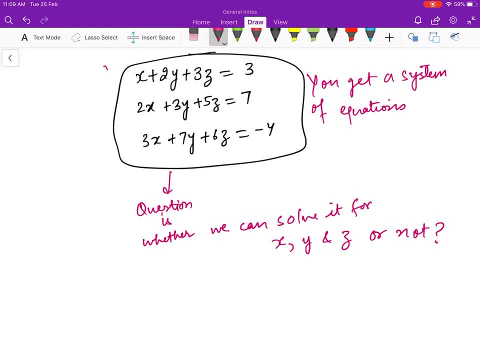 or not. so this is your question, and we know that for such a system, there are three choices: no solution, unique solution- you, and then infinitely many solutions. right, so so we, we just want we this, either of these two cases, we, we don't care whether the solution is unique or infinitely many solutions, all we want is there. 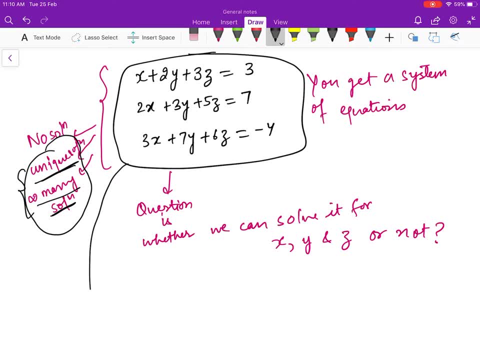 must be a solution. so let us see whether we can solve this system of equations. so there are many ways to solve it. so one of the ways you just write the augmented matrix a, b, that is equal to you write the coefficient matrix one, two, three, two, three, five, three. 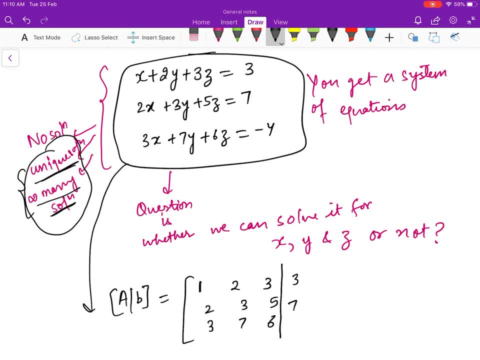 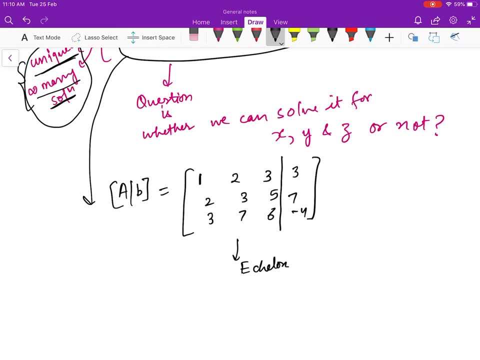 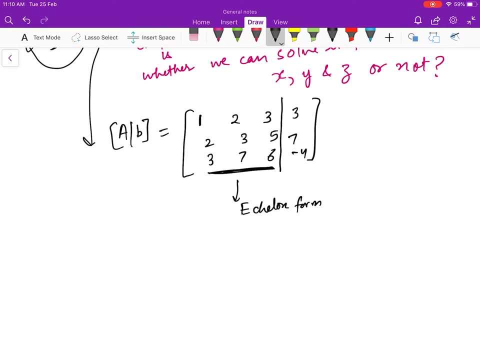 seven, six, and then you just already right inside the 37 minus four. now you can, you can convert it into the echelon form. echelon form means you can make the left inside as an uh, applaud, anglo metric. so we can solve for the x, y that variable easily. so what we can do, we can do like goes to mine- is two times. 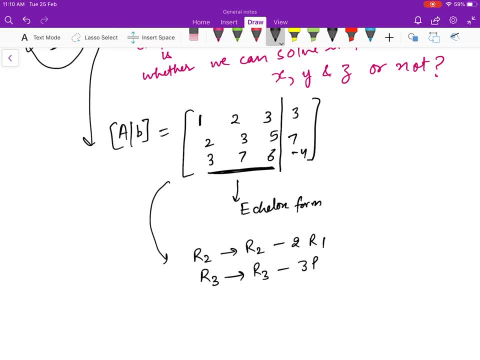 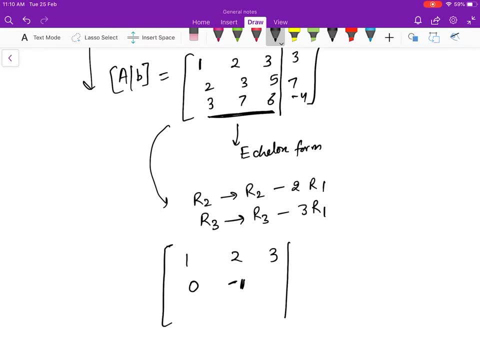 one and three goes to our three min three mix sleep inside R1. so you have 1, 2, 3, then you have 0 here minus 1 here, minus 1 here, and then we have 1 here, 3 here and then you have R3. goes to R3 minus 3 times R1. so it 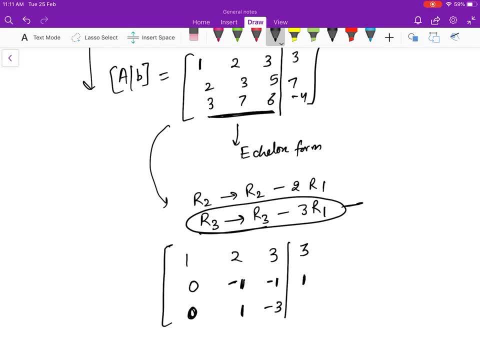 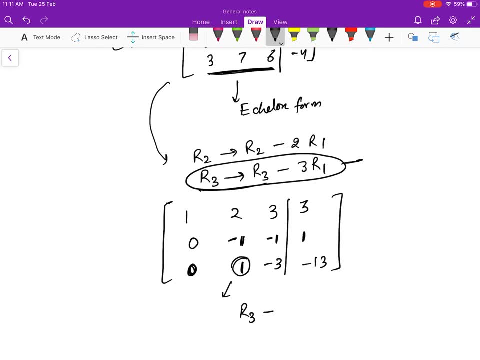 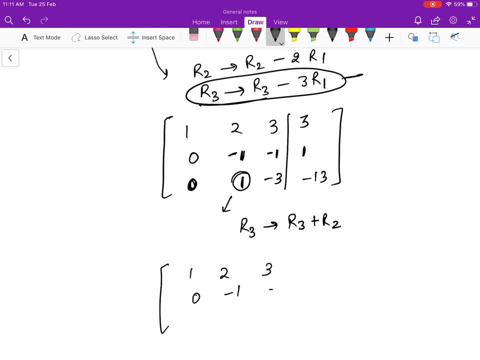 means that you have 0 here, you have 1 here, minus 3 here and minus 13 here. now you want to make it 0. for that you have R3 goes to R3 plus R2. so you have 1, 2, 3, 0 minus 1 minus 1, 0, 0 minus 4. then you have 3: 1 and you have minus 12.